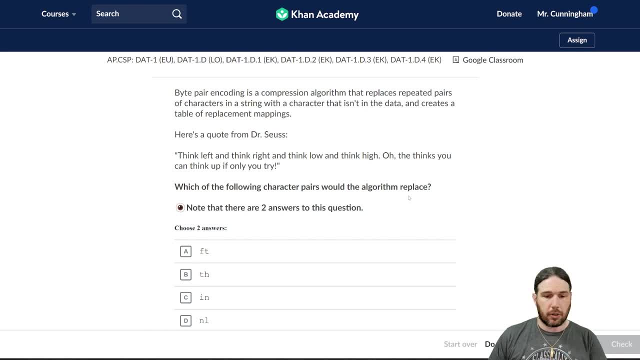 and think low and think right. Oh the thinks you can think up, if only you try. Pretty sure I'm not going to get in trouble for reading that on YouTube. Which of the following character pairs would the algorithm replace? So we're looking for a pair of letters that shows up a lot, because the more it shows up, 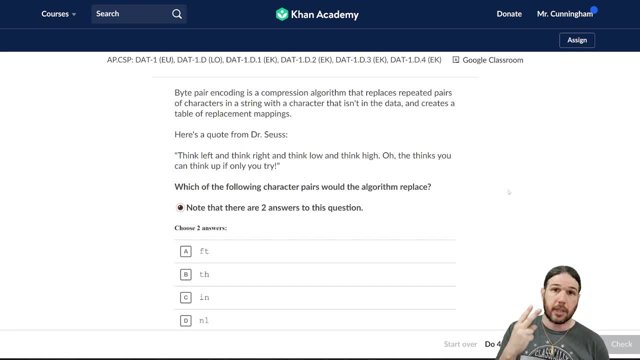 the more we compress it when we replace those two characters with just one character. Note that there are two answers to this question. Well, automatically, I think that T-H is going to be one of the big ones, right, Think low, think high the thinks you can think up. 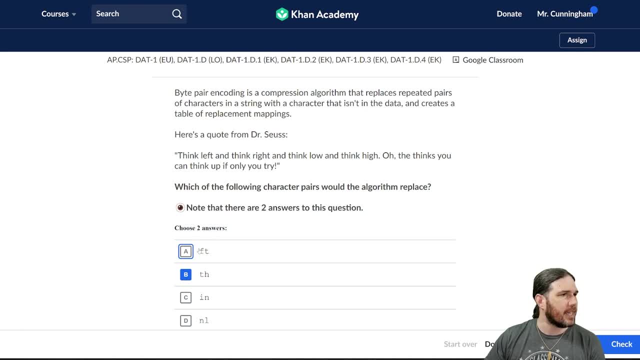 yeah, that's a big one. F-T really only seems to show up in the word left, so I don't think that's really it. I-N- well, I-N is also part of the word think right, So it shows up an awful lot, So that's probably the right. next one, In fact. 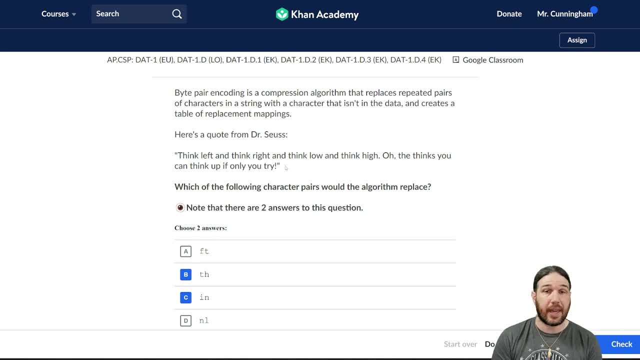 we could probably just have one symbol to represent the word think, and that would take care of a lot of the words, care of a lot of the work for us. How about NL? I don't really see a whole lot in the way of NLs. 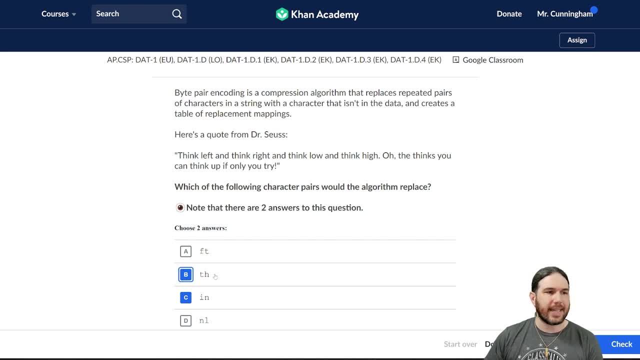 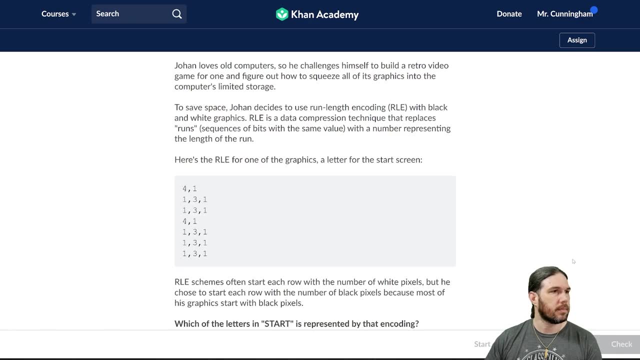 In fact, I'm not sure that I see any at all. So yeah, TH and IN are, of these four options, the best ones. Johan loves old computers, so he challenges himself to build a retro video game for one and figure out how to squeeze all of its graphics into the computer's limited storage. 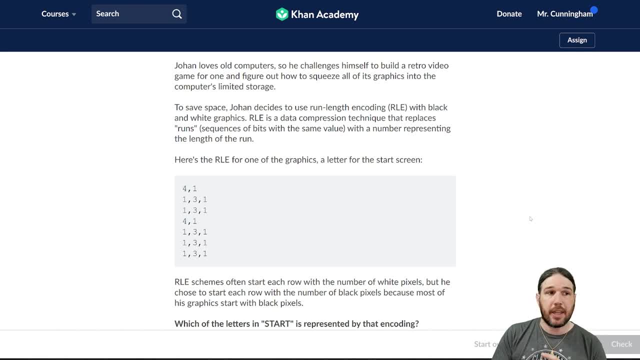 To save space, Johan decides to use a run length encoding with black and white graphics. RLE is a data compression technique that replaces runs, sequences of bits with the same value, with a number representing the length of the run. So in other words, that 4 at the beginning there doesn't represent the length of the. 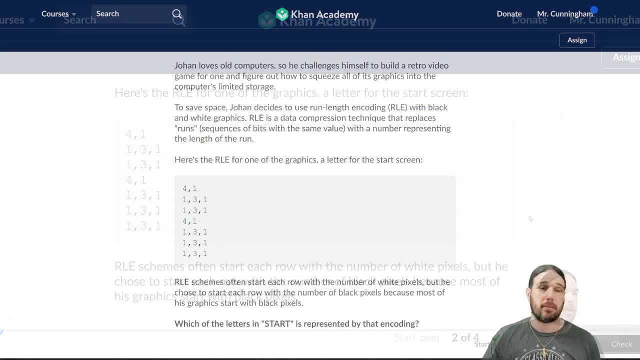 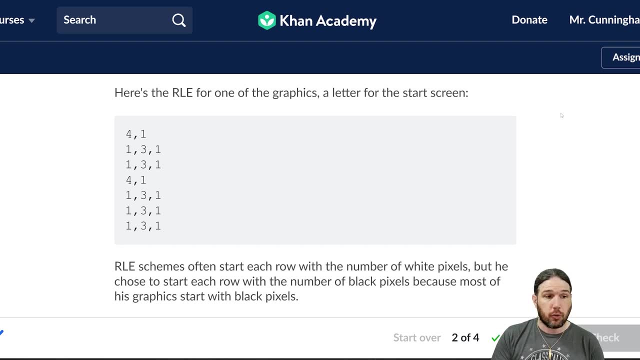 run. It doesn't represent a single color. It means the same color four times. Here's the RLE for one of the graphics, a letter for the start screen. RLE schemes often start each row with the number of white pixels, but he chose to start. 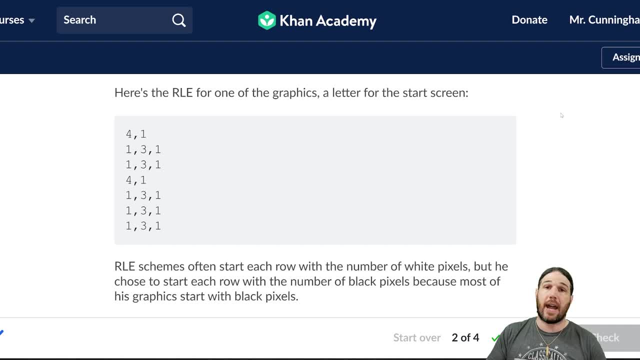 each row with the number of black pixels, because most of his graphics start with black pixels. So what this is saying is: on that top row, there is four black pixels, followed by one white pixel. Same deal in that second row: One black, three white, one black. 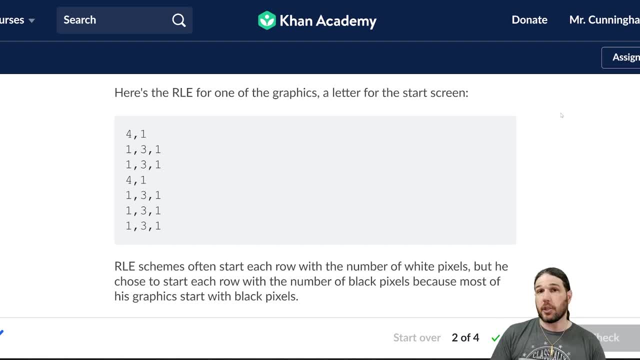 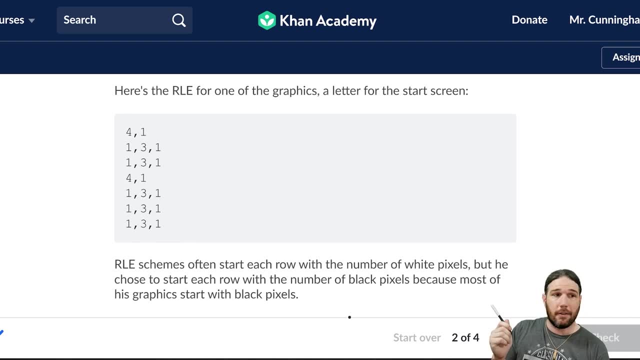 I think I know what this is going to be, but let's go ahead and draw it out just to see. Now, if you look at the shape of that, you can actually probably get a pretty good idea of what the letter is. I don't know if that's coincidence or not. 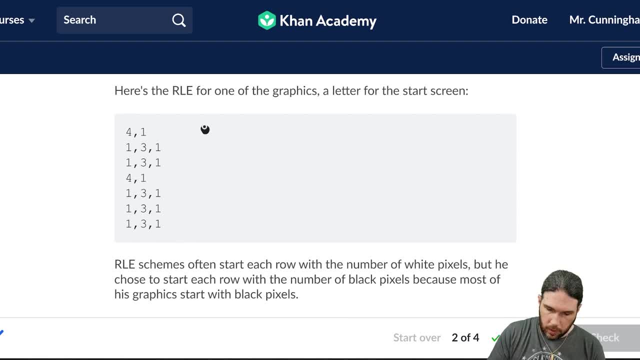 Anyway, let's give this a shot. So it starts out with one, two, three, four black, one white. Yes, I know, pixels are squares and I'm not doing them perfectly. in order, Again, work with me, I'm sure we'll figure it out by the end. 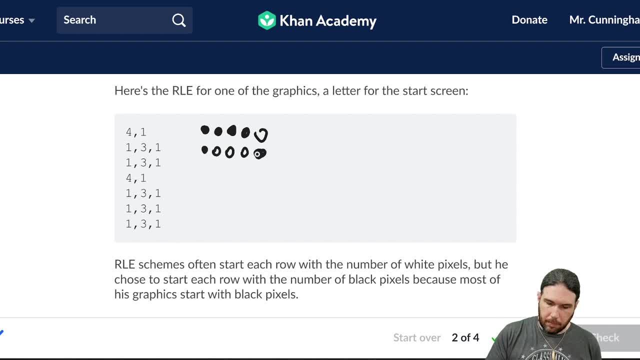 One black, one, two three white and one black. Again one black one, two three white and one black One, three one. I don't know about you, but that looks like an R to me. 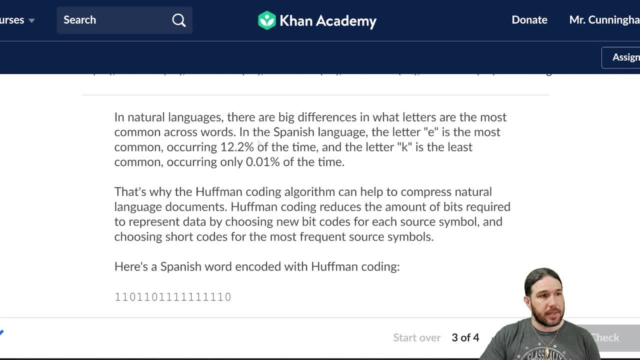 Moving on, In natural languages there are big differences in what letters are the most common across words. In the Spanish language, the letter E- or E, I suppose- is the most common, occurring 12.2% of the time. 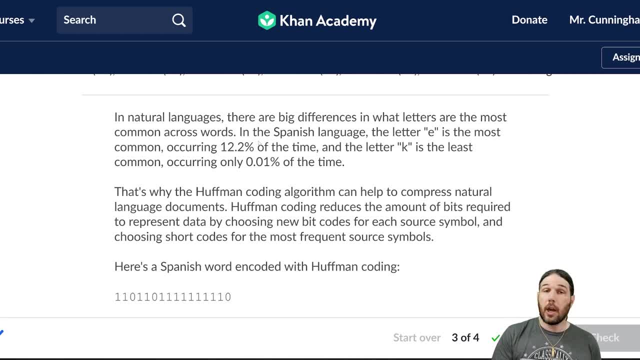 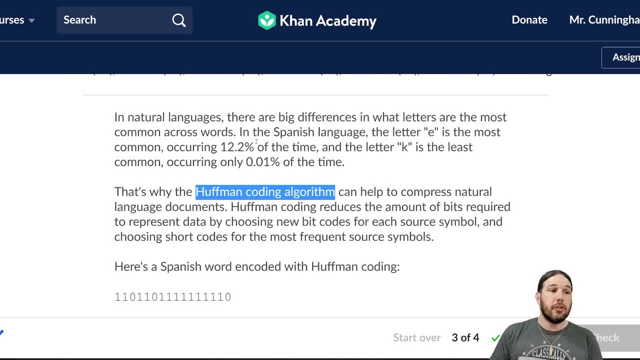 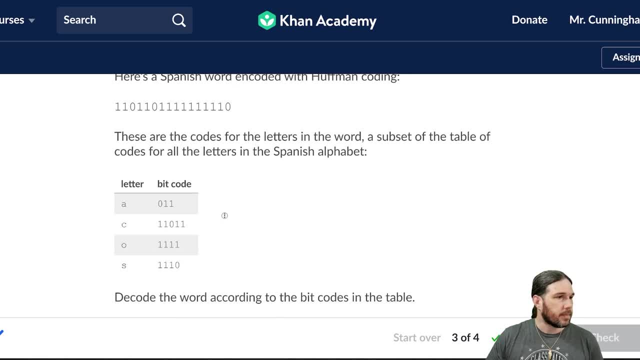 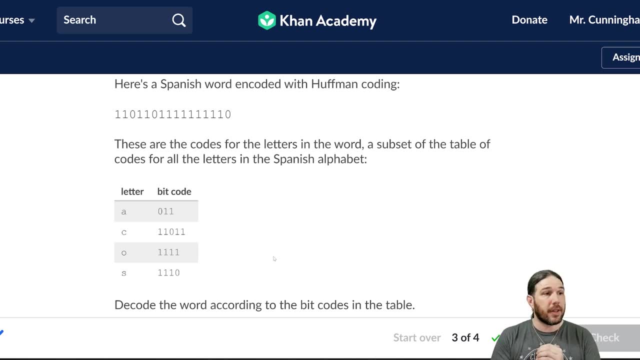 on and see if we can figure it out. Here's a Spanish word encoded with Huffman coding. These are the codes for the letters in the word, a subset of the table of codes for all the letters I see, So it looks like the most common letter. 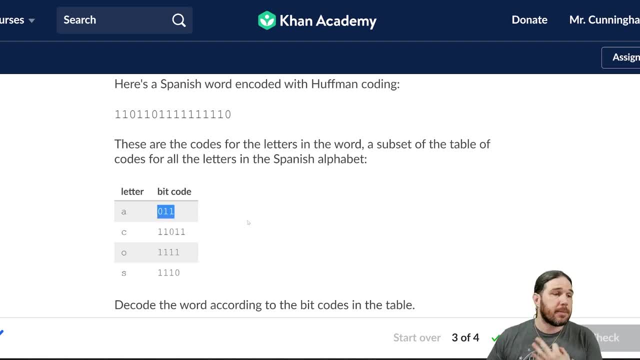 In this case, A only has three bits in its bit code, as opposed to C- which I assume is much less common- has five bits in it. That way you're minimizing the amount of space that each word requires by taking the most.